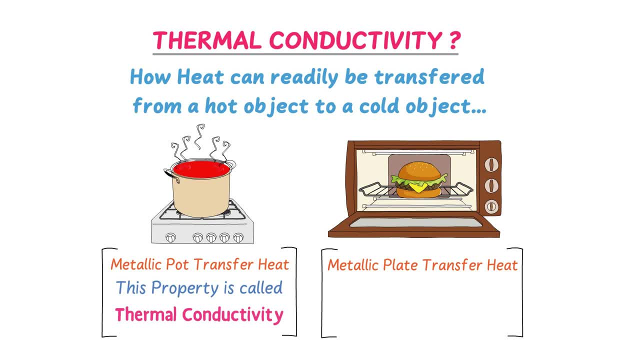 again. the metallic plate absorbs heat and transfer it to the food. So this heat transferring to the food is called thermal conductivity. This property is known as thermal conductivity. Thus we learned that thermal conductivity means how heat can readily be transferred. Now let me teach you that many students misunderstood. 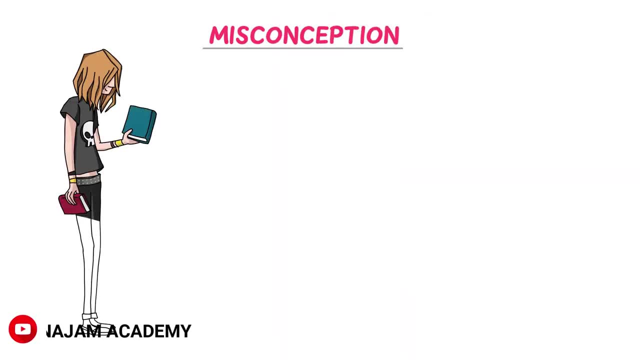 the concept of thermal conductivity. You should note it down. this example: Consider a hot object and a cold object. Now if I connect these two objects using a metallic rod, heat will transfer through this metallic rod. Now let me teach you that many students misunderstood. 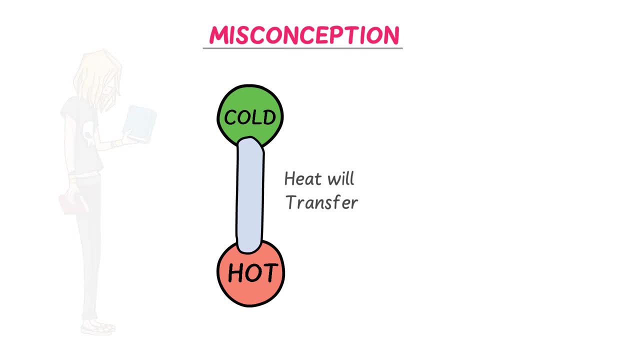 the concept of thermal conductivity. This property is known as thermal conductivity. So this transferring of heat or heat conduction through the metallic rod from the hot object to the cold object is called thermal conductivity. Let me repeat it: This transferring of heat or heat conduction through the metallic rod from the hot object. 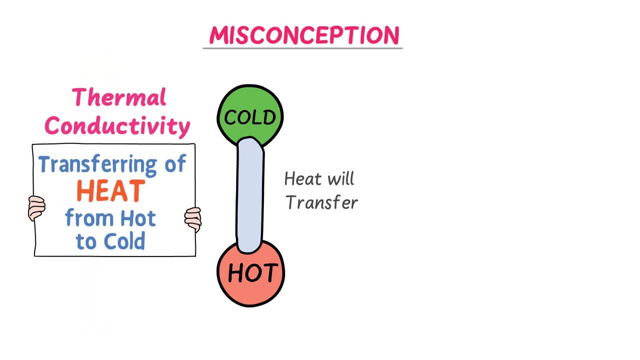 to the cold object is called thermal conductivity. Remember that different objects have different properties. Now let me teach you that all the objects with both heat are equal, We will have different thermal conductivity. For instance, consider these same hot and cold objects. 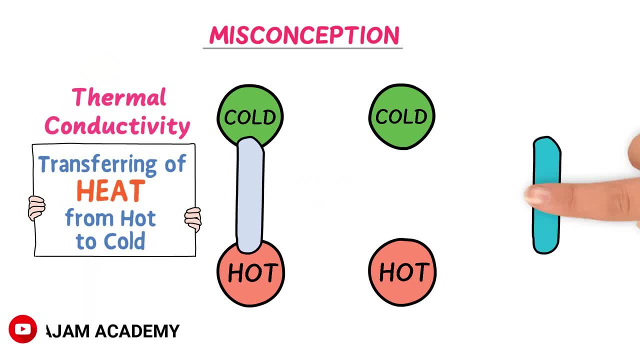 This time, instead of metallic rod, I insert plastic rod between them. We will observe that comparatively less heat will transfer from the hot object towards the cold object. Thus we therefore say that metals like this rod have high thermal conductivity, while non-metals, like this plastic, have low thermal conductivity. If you wonder about this difference in thermal 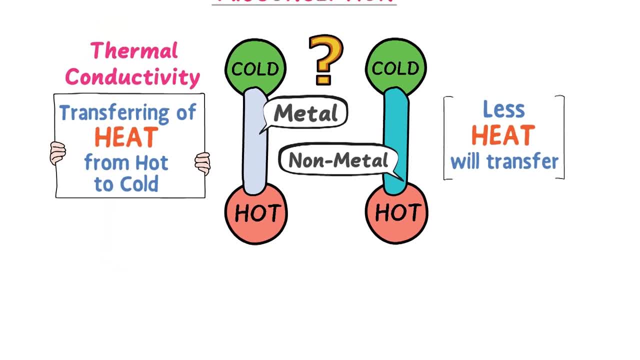 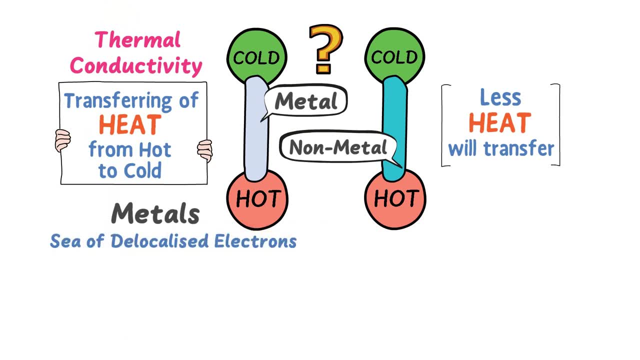 conductivity? then the answer is very simple. Within metals there is a sea of delocalized electrons. Delocalized electron means free electrons that can move from one corner to other corner of the metal. So metals therefore have high thermal conductivity, While non-metals